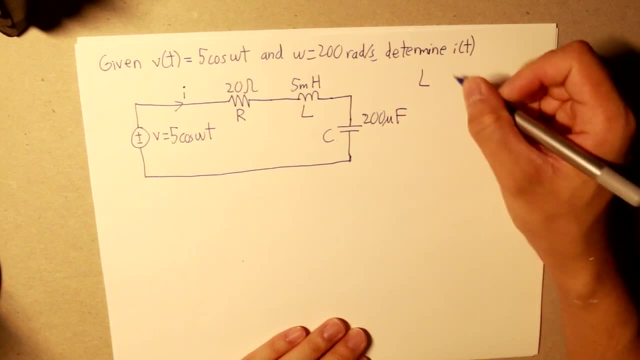 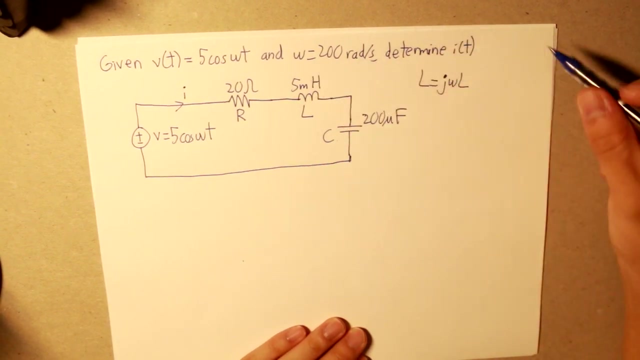 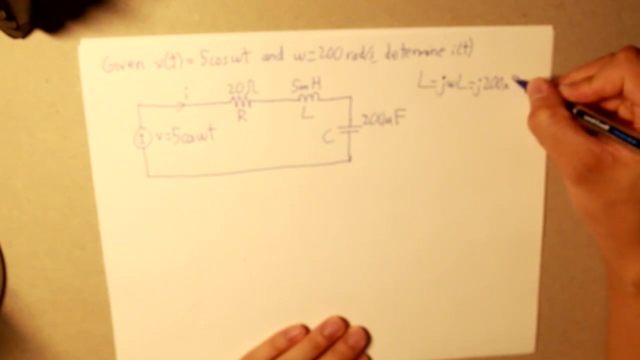 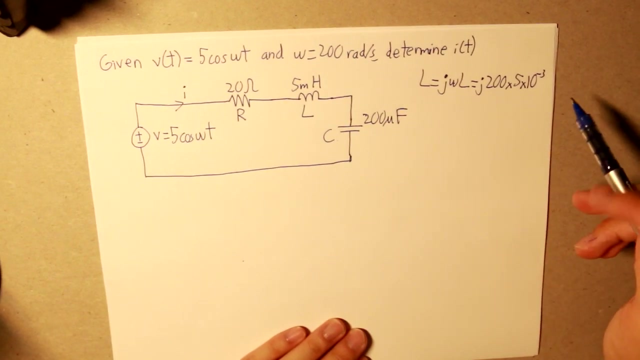 start on our inductance. So our inductance define our ohms. we use the equation J WL. so, given that the angular frequency W is 200, so we have 200 here. what we get is J times 200 times 5 times 10 to the negative three. this is mila. So we get that and our answer to that. 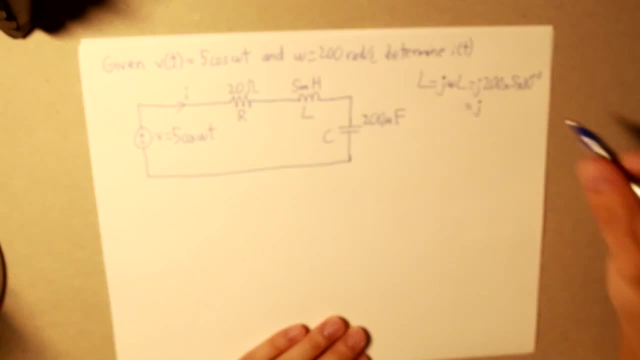 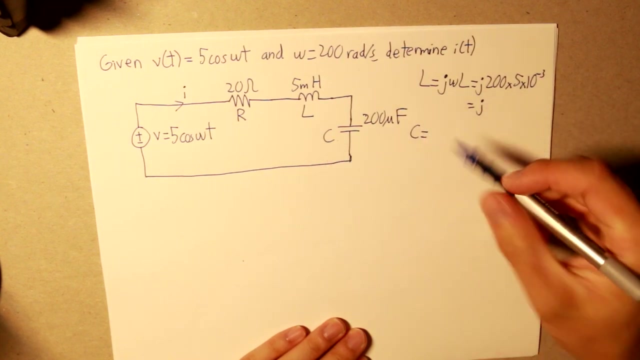 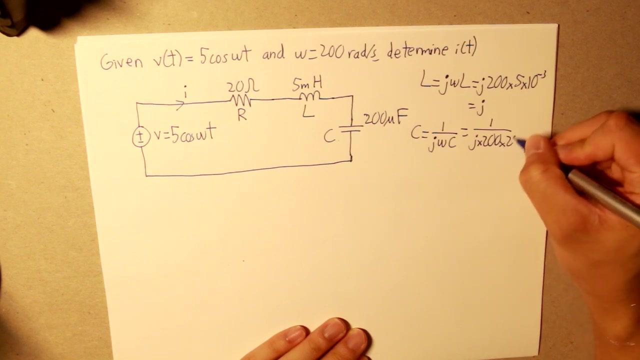 will be one. so we have J alone. Now let's go to our capacitor. we know that for our capacitor our equation would be 1 over j times angular frequency times, the capacitor, and that will be equal to j times 200 times 200 times 10, to the negative 6,. and our answer: 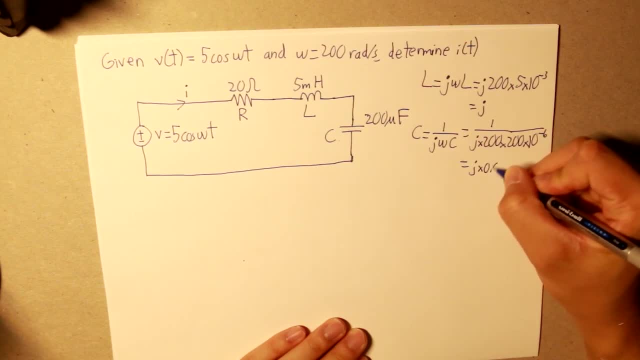 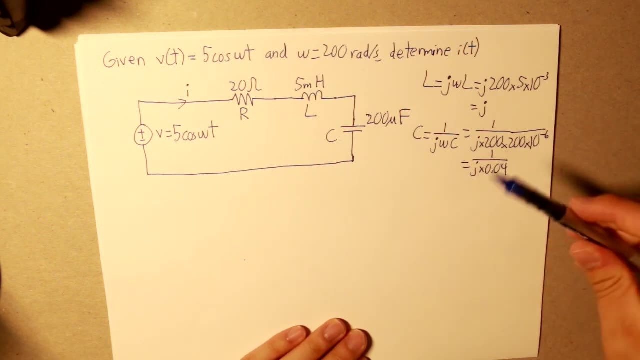 will be 0.04 for the denominator. and now let's put that into the numerator. so since our j is in the denominator, we know by complex identity- that would be equal to negative j. and if we take 1 divided by 0.04, what we get is 25, so now that we got our inductance, 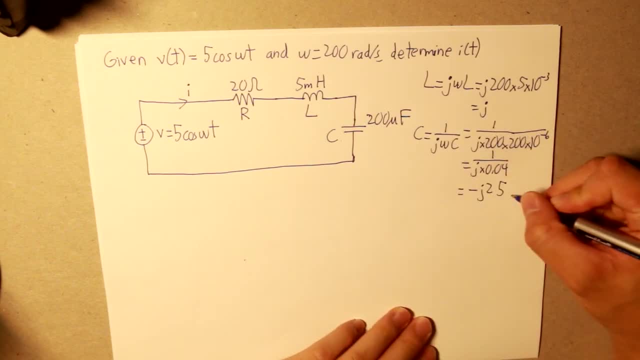 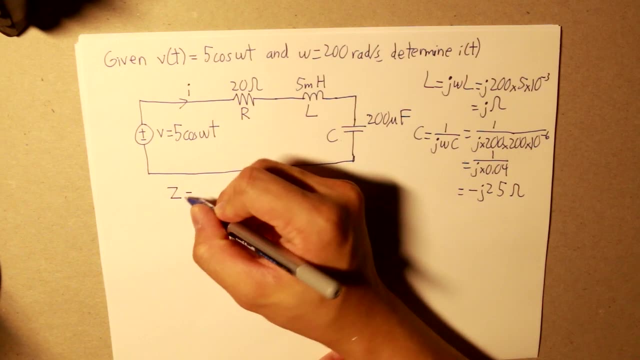 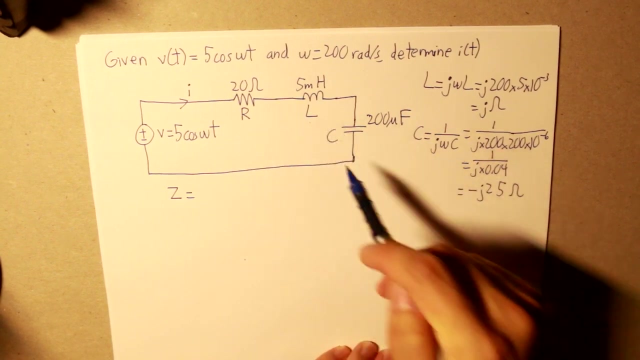 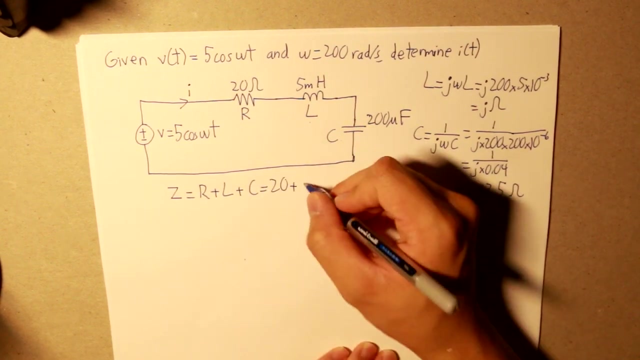 value in ohms. and now that we got our capacitance value in ohms, let's write these in the end term. now we can add up the total impedance- now our impedance, as we know, is equal to the resistor Resistor plus the inductance plus the capacitance- and that we get 20 plus j minus j25, and our 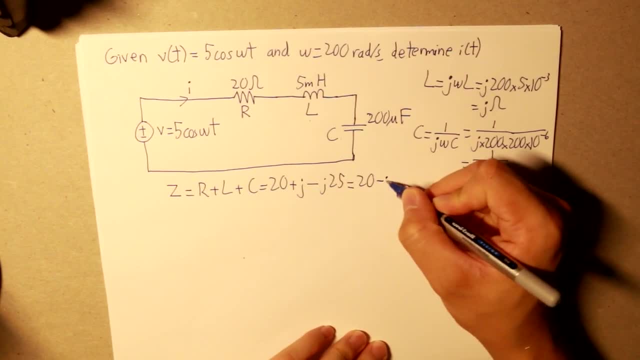 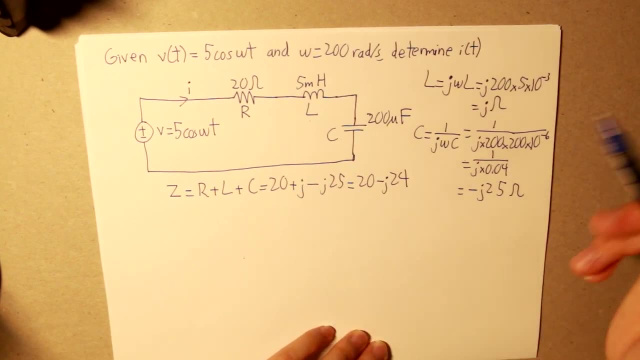 total impedance shall be 20 minus j24.. Now you may be wondering: why did I calculate the impedance? Well, what we know by ohms law, that v is equal to the current multiplied by the resistor. In this case, we have 20 minus j25.. 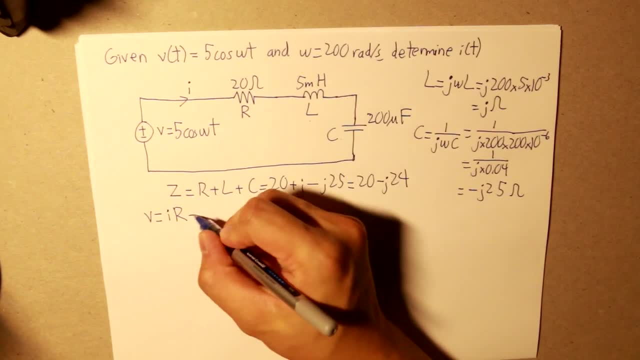 In this case, we have 20 minus j25. In this case, since we have inductor inductance and capacitance, that will be simply equal to the current multiplied by the impedance. and that impedance- well, we just calculated. 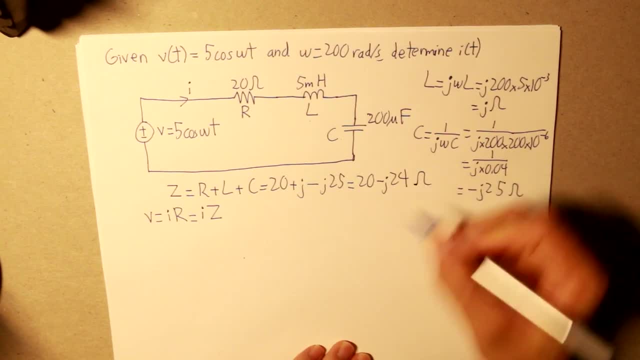 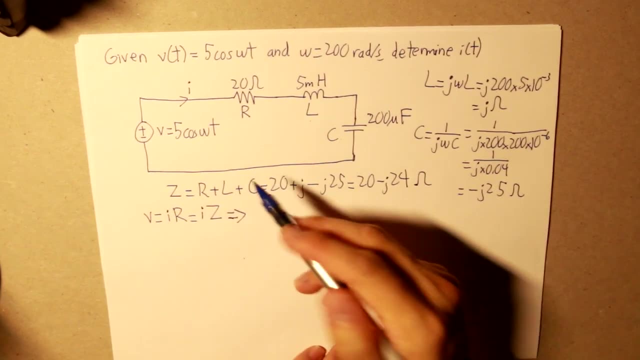 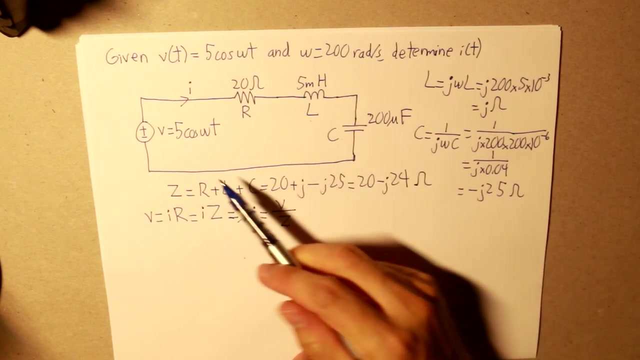 right here. So our current? that's what we're trying to find. we take the impedance and we move it to the other side and what we get is the current is equal to the voltage divided by the impedance. Now, going and moving on to our voltage, 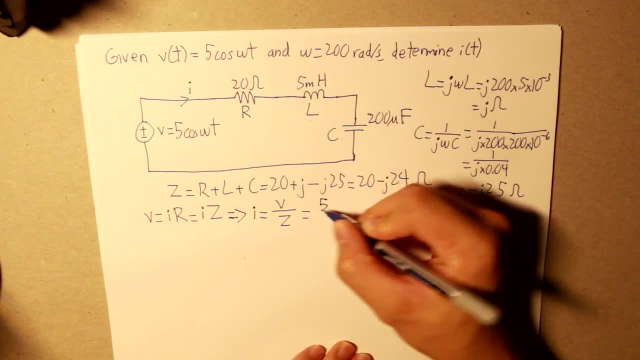 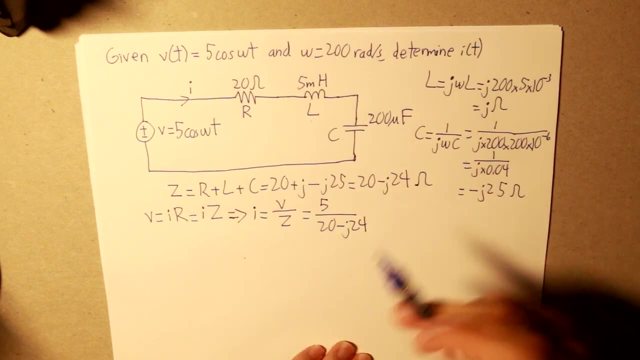 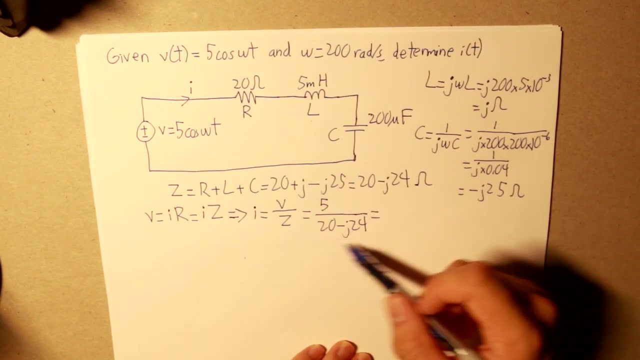 What we do know is that our voltage is 5, and our impedance is this: 20 minus j24.. Now, using the division of simplification, what we're going to do is try to simplify the denominator out, since this looks more complicated than your numerator. 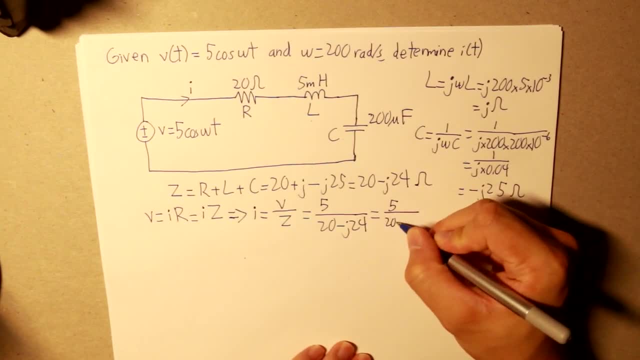 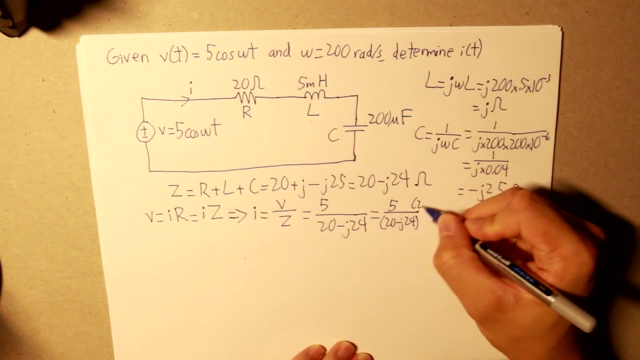 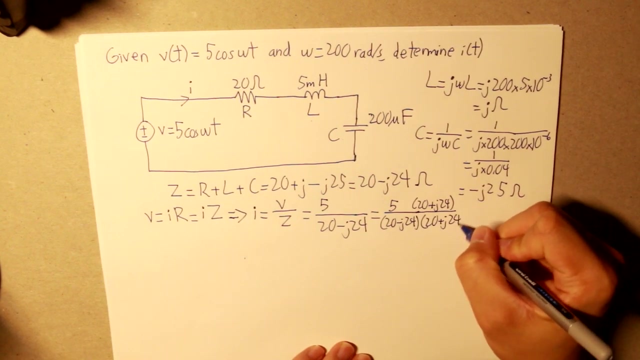 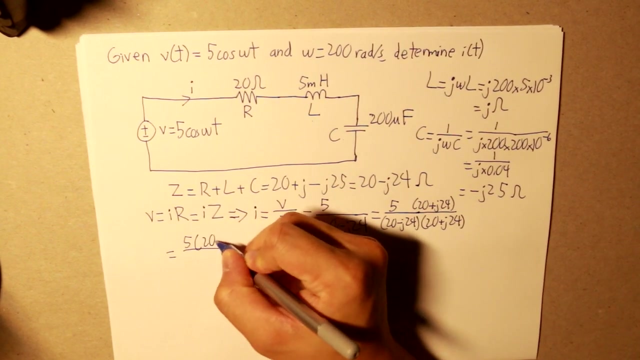 So we have 5 divided by 20j24, and what we're going to do is we're going to multiply 20j24 in the numerator and in the denominator. So what we get in the end is 5 times 20 plus j24, and then we get 20 squared plus 24 squared. 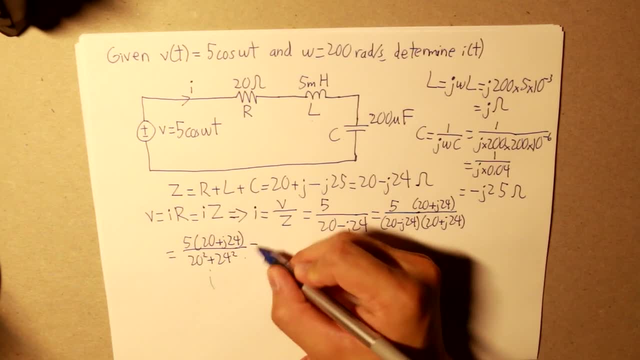 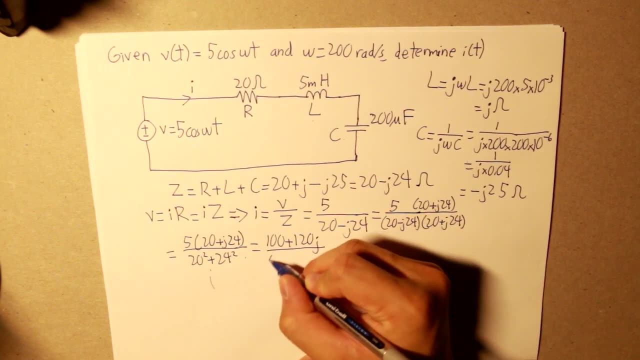 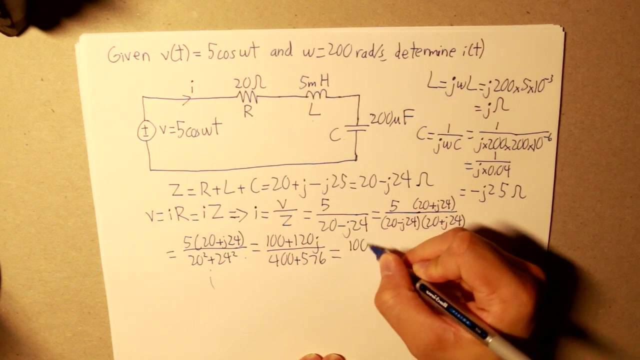 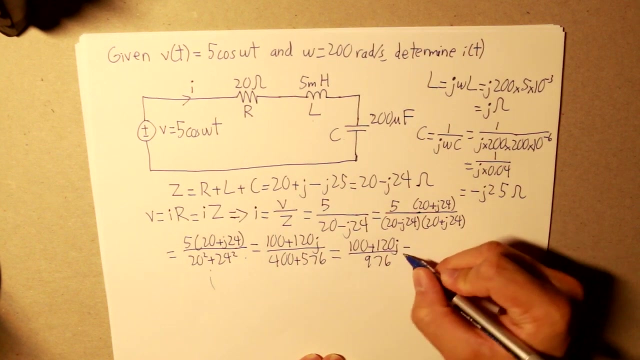 And what we get in the numerator is 100 plus 120 plus j24.. 420J, 400 plus 576.. We simplify them out by adding both terms in the denominator and what we get is 0.102 plus 0.0102J. 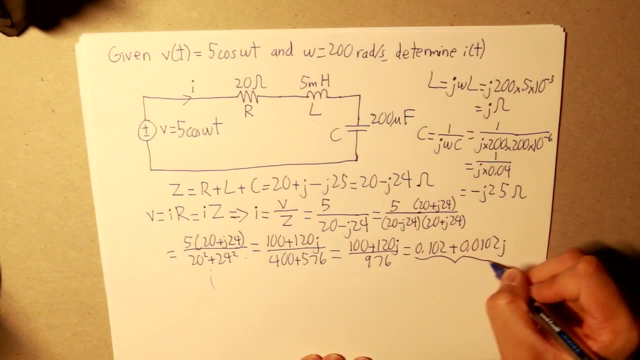 Now you may be wondering: is this the final value? Well, when it comes to circuits, what we want to do is define its polar form. This is the rectangular form, as I've mentioned before in my previous videos. So current is equal to 0.102 plus 0.0102J amps. 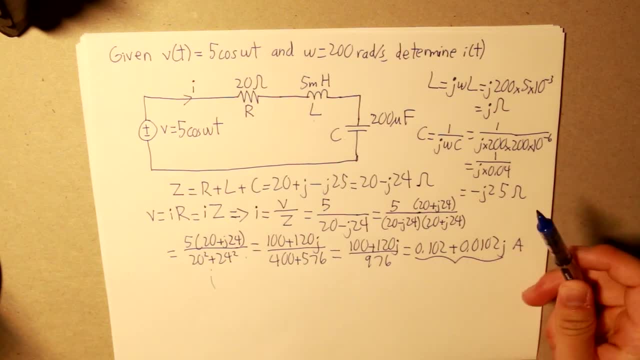 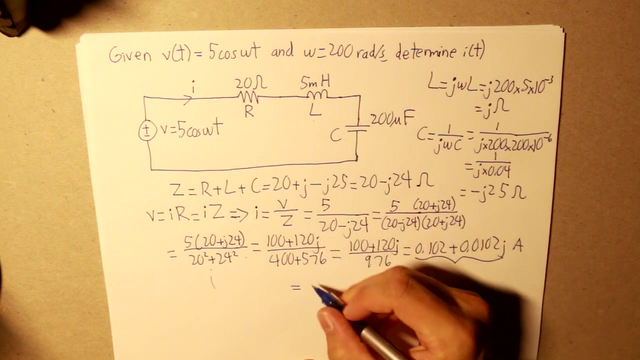 That seems a little complicated for a student, right? So what we need to do is translate that to polar form. First, what we need to do is find its magnitude, Determining the Pythagorean Theorem: 0.102 squared plus 0.0102 squared.